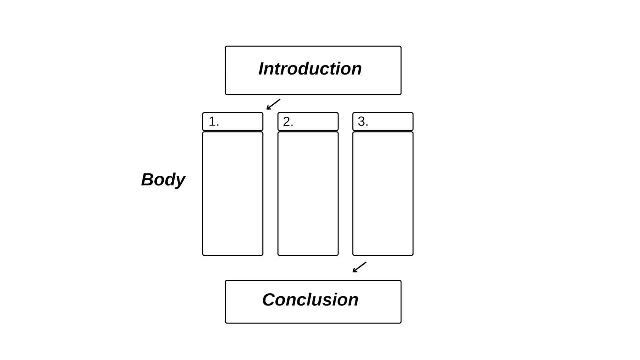 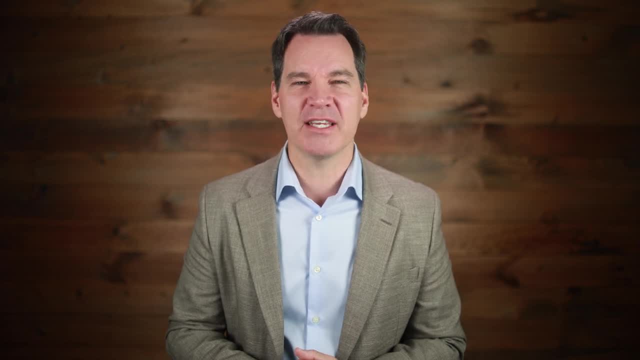 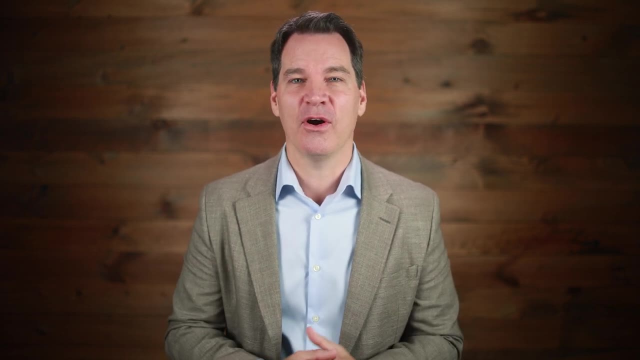 Finally give a clear conclusion. In fact, say the words in conclusion, to signal that you're wrapping up. Quickly recap your main point And you're out. This is the classic public speaking design. for a reason: Don't fight it. Trust that this basic design will work for 90% or more of your messages, especially if you're 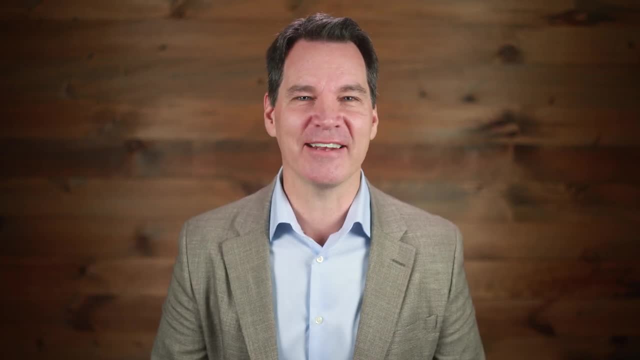 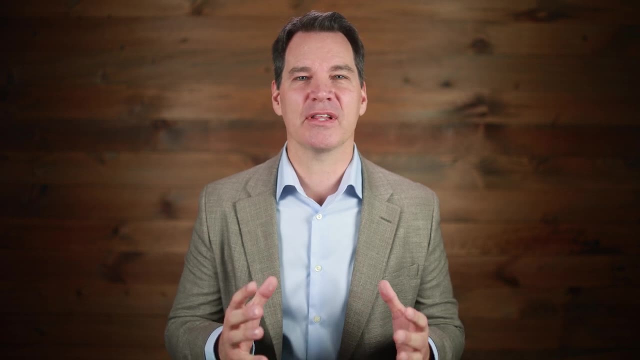 a beginner. Your audience will be grateful that you had a clear plan and they'll remember what you said, which is the whole point of preparing a message like this in the first place. Organizing a message like this takes a little more behind-the-scenes effort and time, but it'll help. 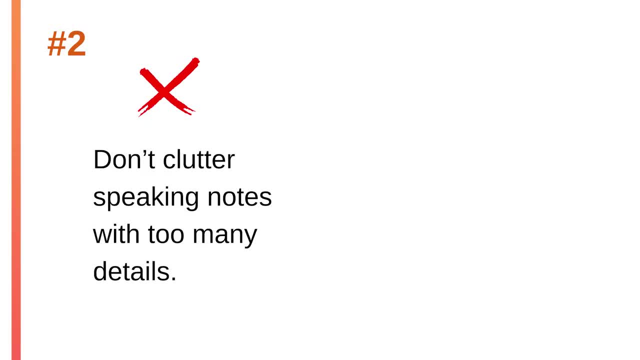 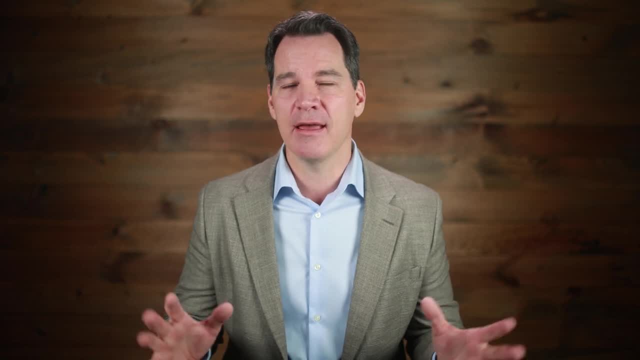 you sound great. Number two: don't clutter. Don't clutter up your speaking notes with too many details. This is another common mistake. We're often tempted to pack our notes with everything we want to say, and that's natural, because we don't want to forget, But when it comes to the actual presentation we'll get. 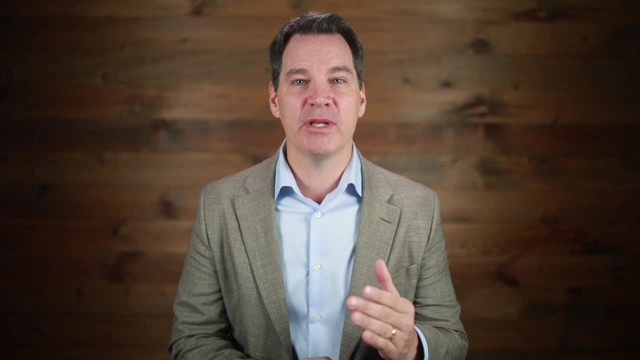 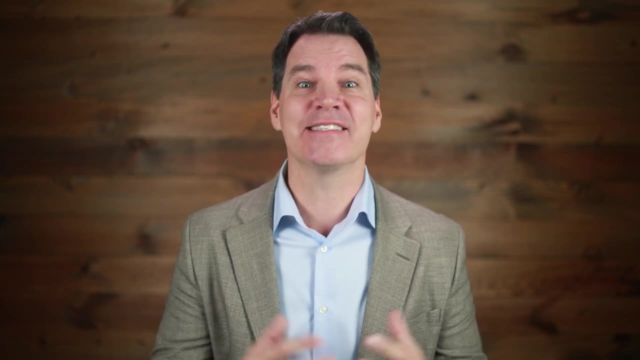 nervous in the moment And the most likely outcome when we have too many notes is just to lock in on our notes and look down the whole time. We end up reading essentially and we sound like we're reading. It comes across as stiff, wooden and robotic and it pretty much ends up being a 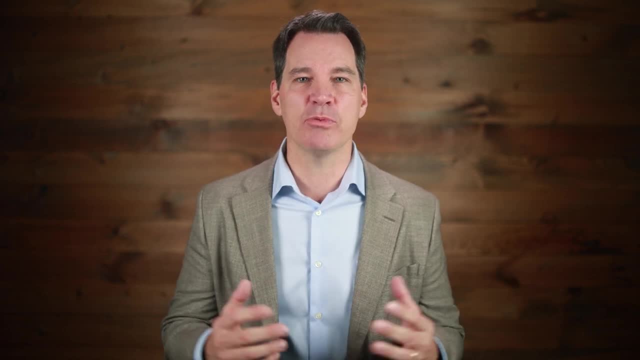 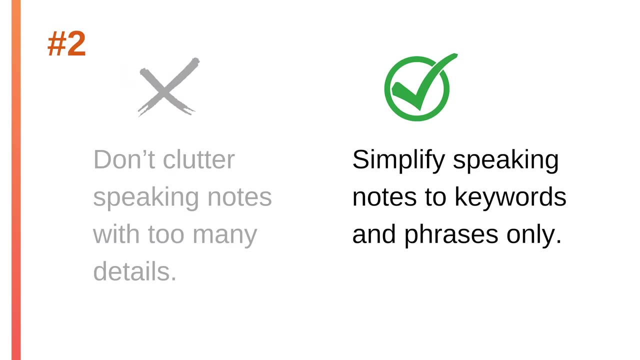 mess. Instead, pare down your notes as you practice so that you can have a structured conversation with your audience. Your goal is to have just key words and key phrases on your note cards. We call these talking points. I have a whole video about how to whittle down your notes. 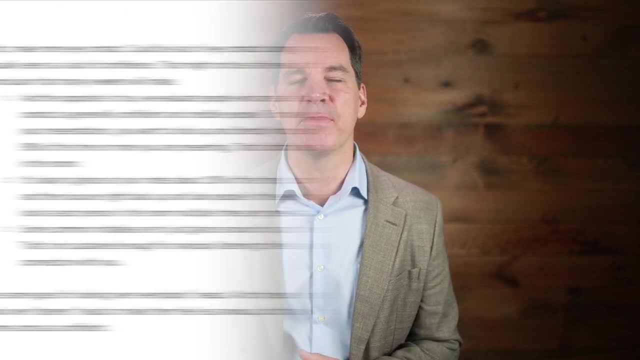 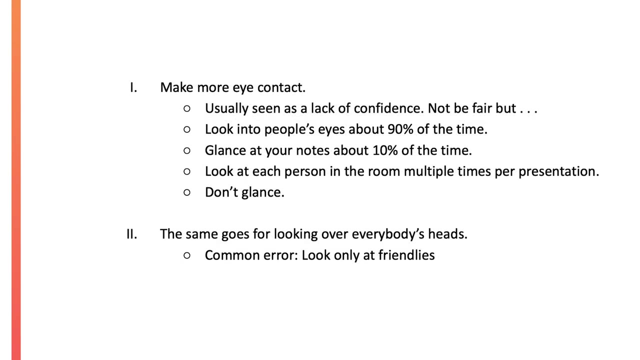 as you practice. I'll put a link to that in the description below. The short version is: practice a few times, cut your notes in half. Practice a few more times. cut your notes in half. Do this over the course of a few days so that by the time you're ready to go, you're going to be able to. 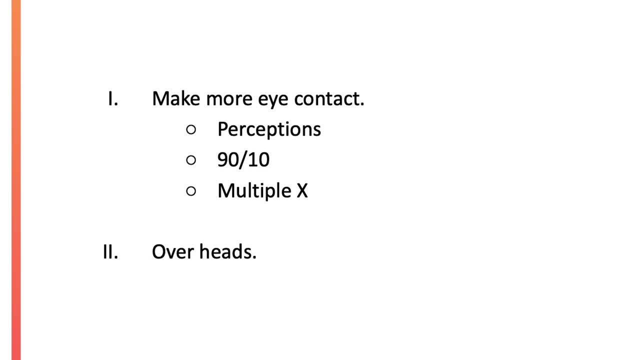 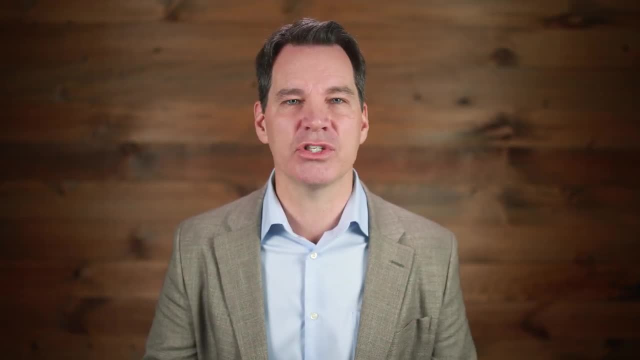 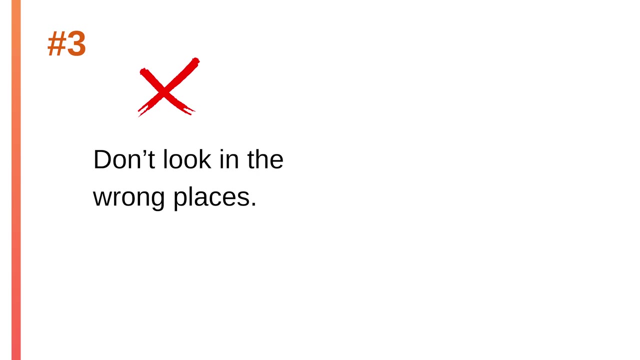 stand up and speak. You have simplified notes with key words only. You can just glance down, see what's coming next. look up, connect and have a comfortable conversational style where your personality shines through. Using simplified notes is freedom. Number three: don't look with. 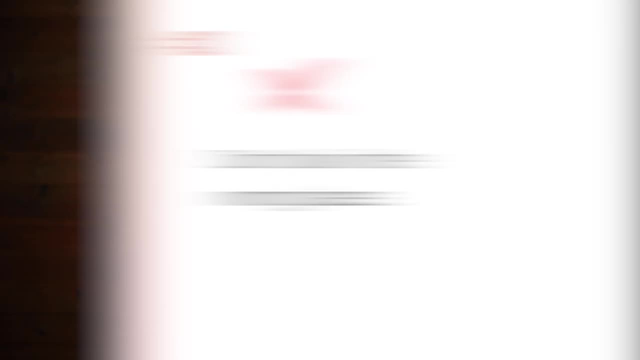 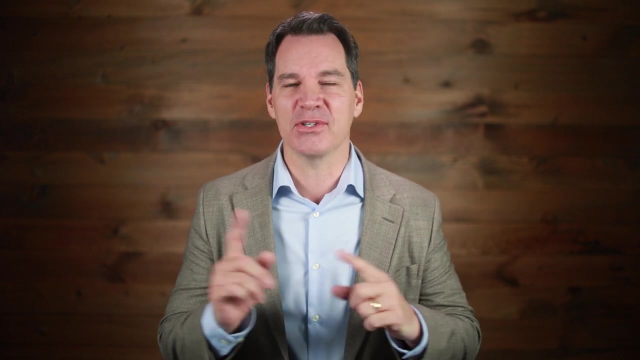 your eyes in the wrong places. Here's where not to look. Don't look over listeners' heads. That's terrible advice I've heard many times. Don't look at the floor, Don't look at the ceiling or dart your eyes in the wrong places. Don't look at the ceiling or dart your eyes in the wrong places. 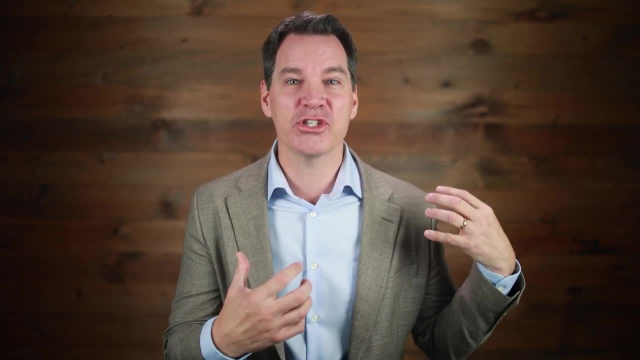 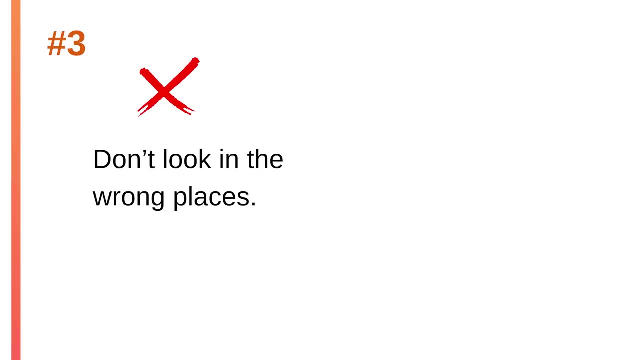 And, for goodness sake, don't turn your shoulders and look back at the screen. Nobody wants to watch. you read right from the slides. So here's what you should do: Look directly into each person's eyes long enough to finish a thought and then move on and look directly into the next person's eyes. 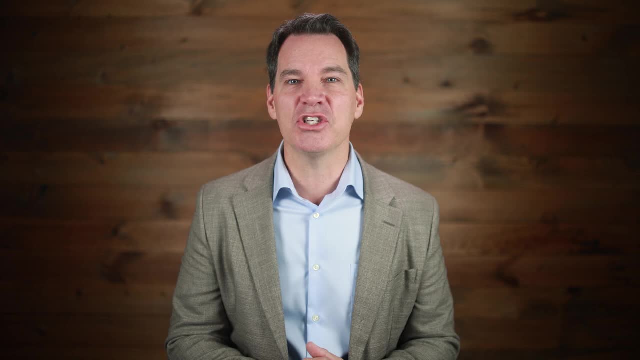 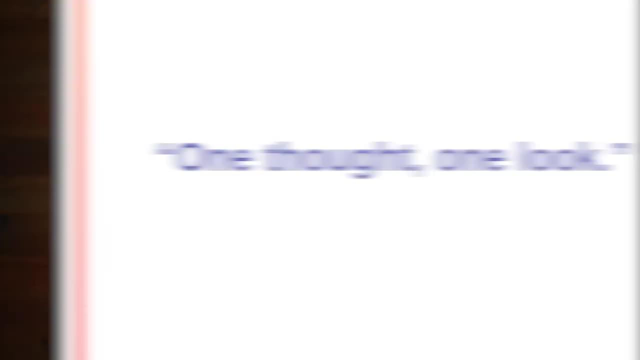 long enough to finish a thought. I've said it in other videos. a teacher once said that eye contact and public speaking should follow this pattern: One thought, one look. In other words, make eye contact for about a half a sentence or so and then move on to the next person. One thought, one look. 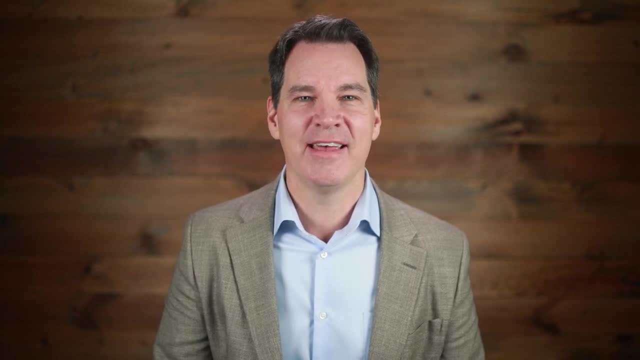 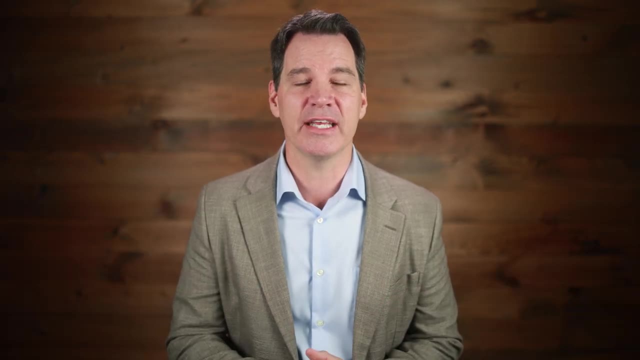 This is about three to five seconds for each person at a time- and make it your goal to look at each person in the room a few times during your presentation. I'll admit this is easier said than done. It can feel awkward to look right into people's eyes if you're not used to it, But 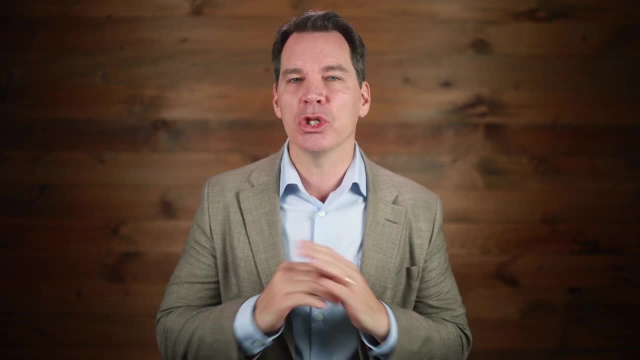 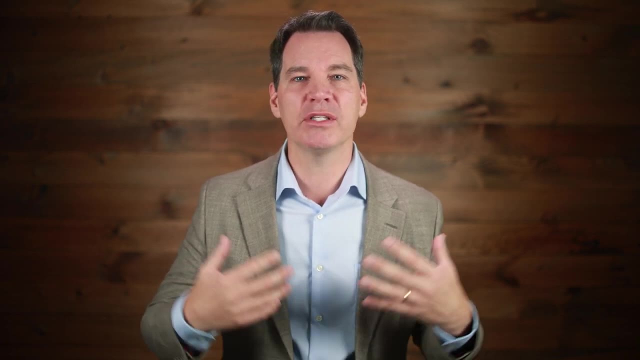 remember you're doing it for your listeners. If you don't look them in the eye, they won't feel like you made a connection with them, And listeners want the fact that you're doing it for them. They feel connected. They want to feel part of the process when you are the speaker. 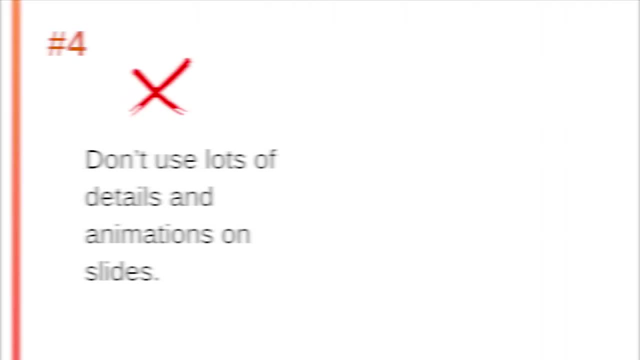 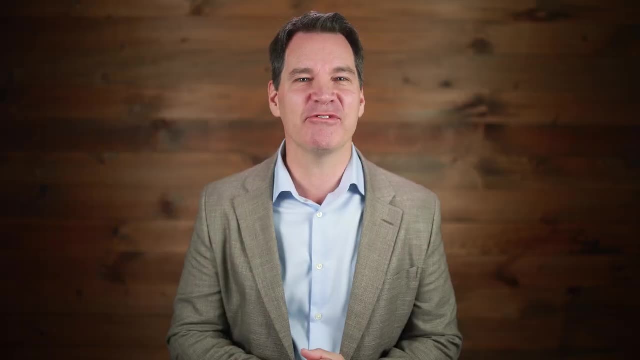 And if you don't make eye contact, your message won't sink in as much. Number four is similar. For the same reasons, don't load up your slides with too much text or animation, As mentioned. if there's too much on your slides, you'll be tempted to look back. 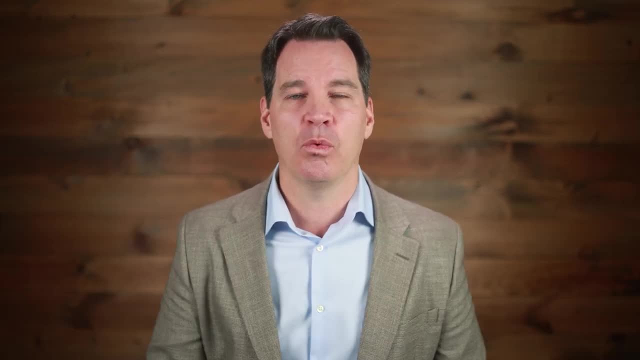 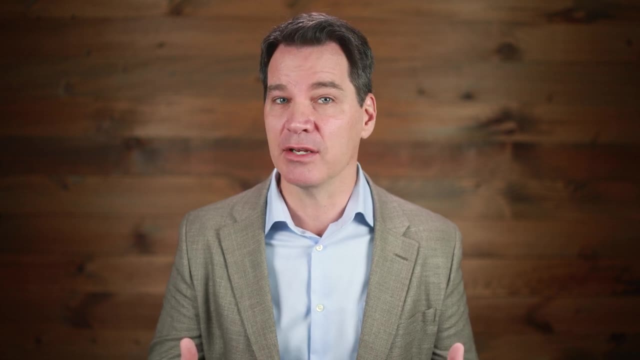 and read from your slides or explain everything that's on there. Once you turn away from your listeners like this, you'll lose all engagement. And some people think that their slides are their speaking notes And then they're not. And some people think that they're not, And some people. 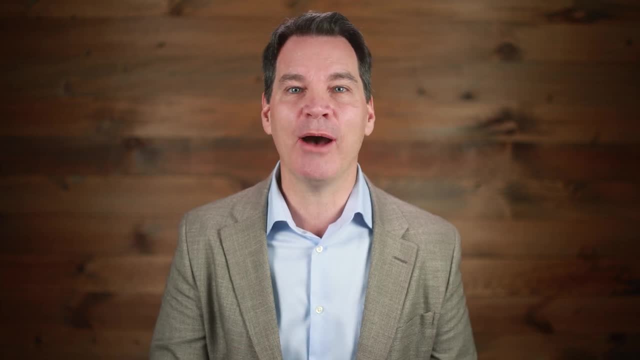 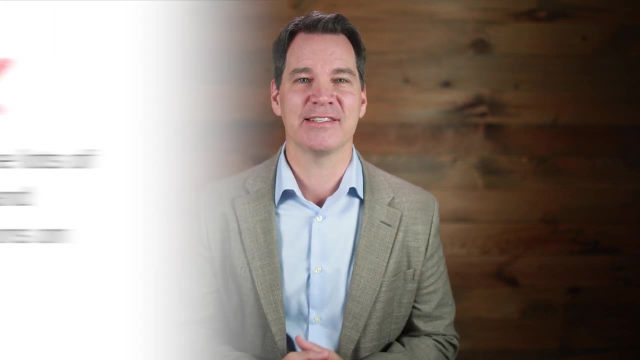 rely on them. Essentially, they can't do their presentation without looking back at their slides, And all of that detail and text will make it difficult for your listeners to understand what's on your slides as well. Instead, make sure your slides are clear, simple and help you make. 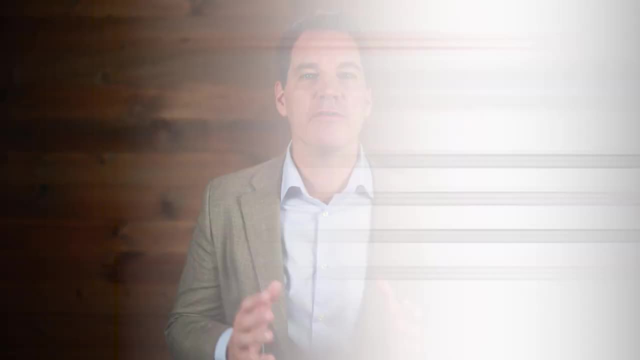 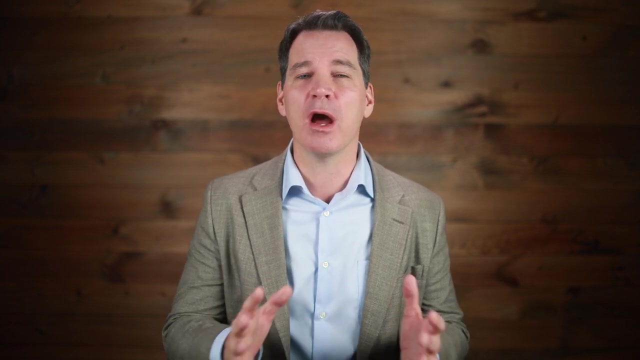 whatever point you're making at that particular moment. A rule of thumb I like to use is that if you're spending more than two or three minutes on each slide when you're preparing them, then you're probably wasting your time. Beginners tend to over-rely. 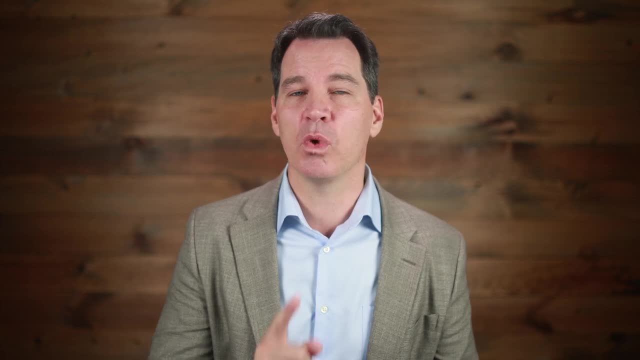 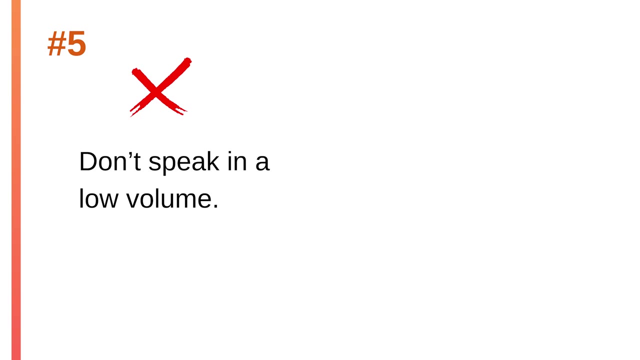 And use too many slides. Don't use more than one slide per minute as a maximum Number five. don't speak too softly or in a low volume. Most beginning presenters speak too softly. They're only loud enough so that the people in the front of the room can hear them. 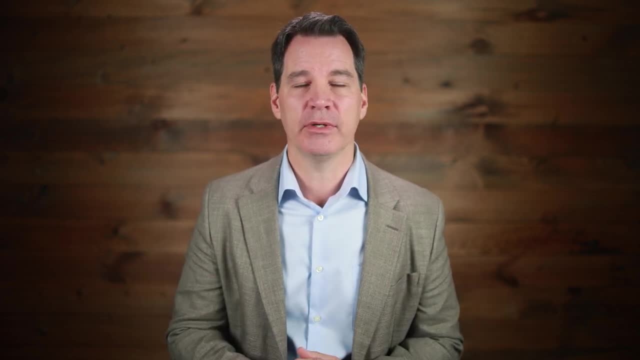 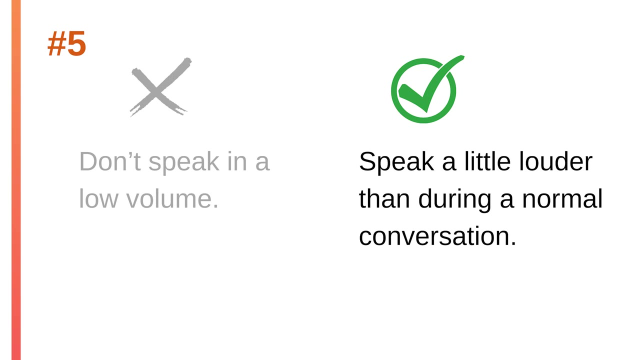 People further back won't be able to hear you in a low volume And it won't make you sound confident to speak like that. So a key tip is to speak a little louder than you usually do in a conversation. Your voice should fill the room. 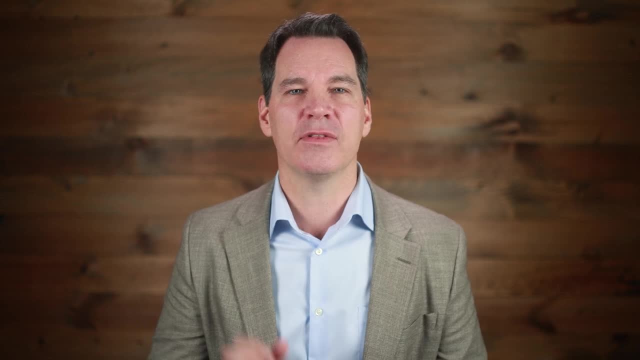 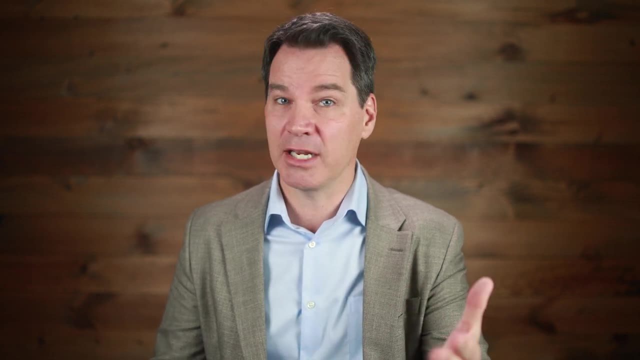 No, you're not yelling. You're just projecting your voice all the way so they can hear you. in the back row, I usually pretend when I'm speaking that the people in the back row have a slight hearing loss, which many people do. If you think of your voice as an old-fashioned 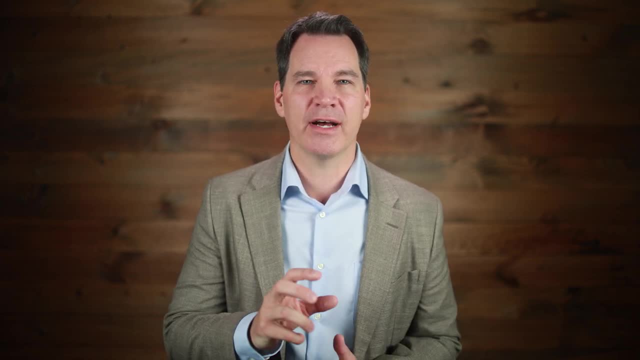 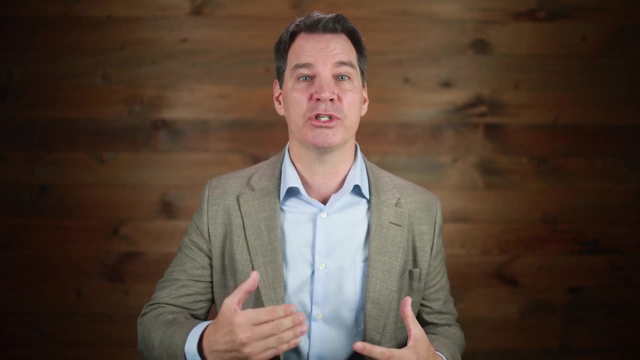 volume knob on a radio. move your volume from five or six up to about seven or eight. It may feel awkward at first but you have to speak in a confident voice if you want to project that confidence to your listeners. Number six: don't fidget with your feet. 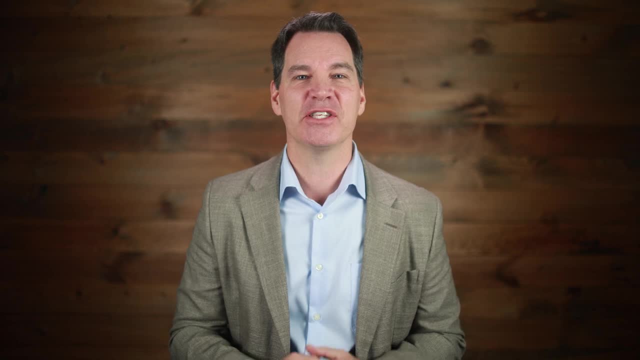 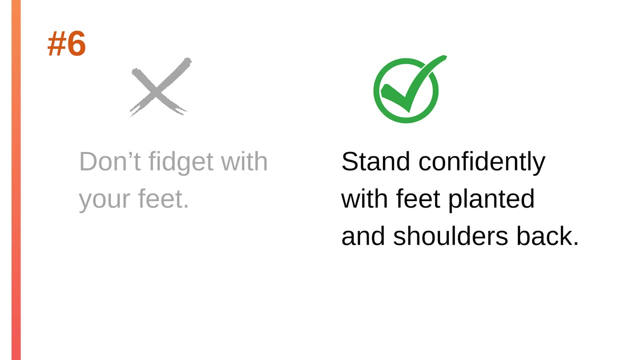 don't pace back and forth aimlessly because you're nervous. This will distract your listeners and it'll make you look anxious. Instead, for your posture, stand confidently in one place with your shoulders back and square. Stand there for a little while and then, if you want to move, move with a purpose. 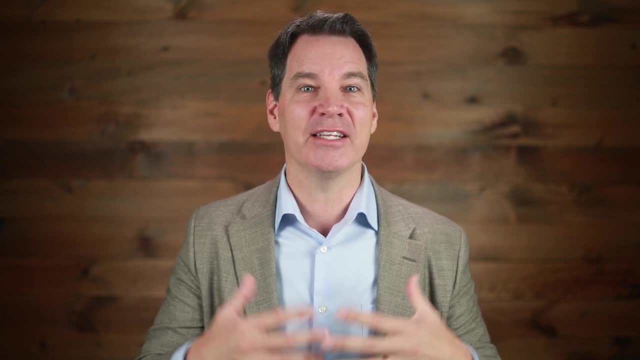 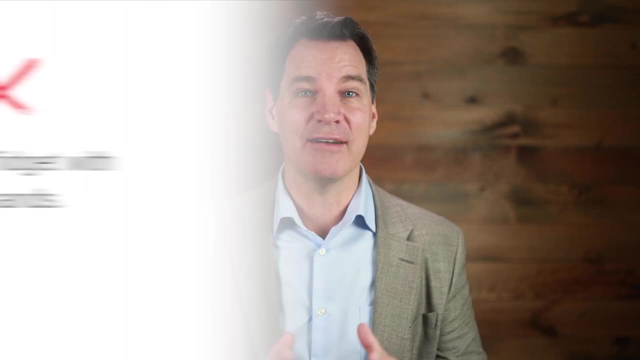 Take a few steps and then stand firmly in another place for a while and share another part of your message. That kind of feet planted stance and posture will make you look prepared and confident. Number seven: don't fidget with your hands. You don't want to put them in your pockets. 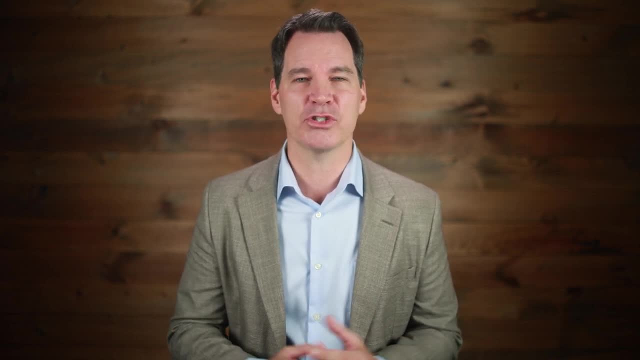 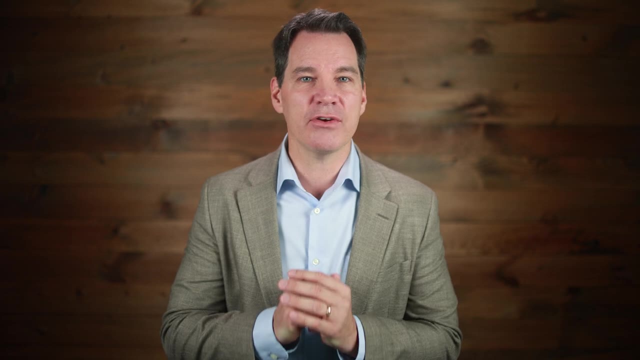 for example, or play with a pen or do anything else weird or distracting like that. You want to use small gestures that emphasize your ideas As you practice your presentation. just let your hands go and gesture comfortably as you rehearse. Practice small little gestures, just like this. 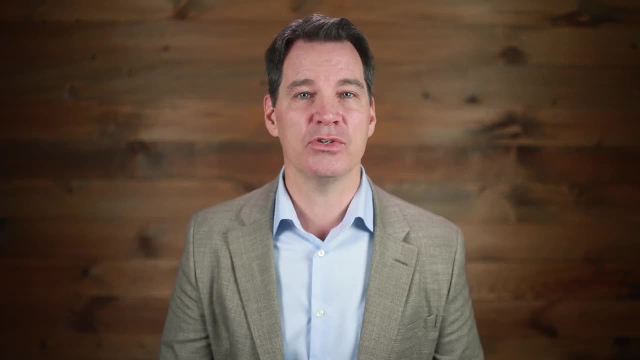 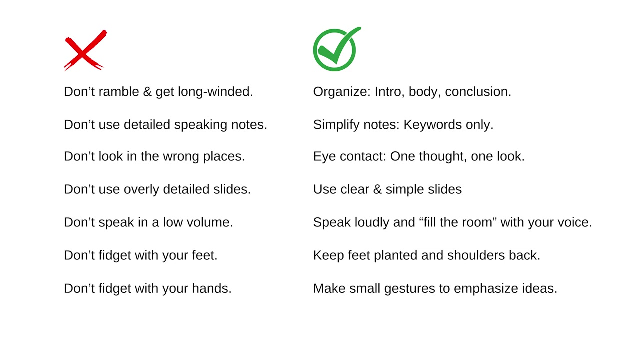 Simply open your hands on the most important word of each sentence or two. Practice like this and it'll become second nature and relaxed during your actual presentation. Here's a quick summary of all seven do's and don'ts. Feel free to leave a comment about the.